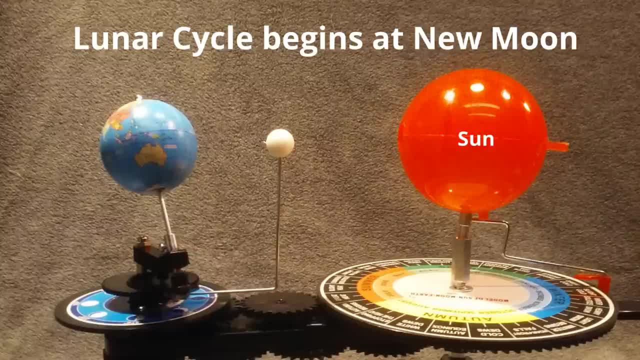 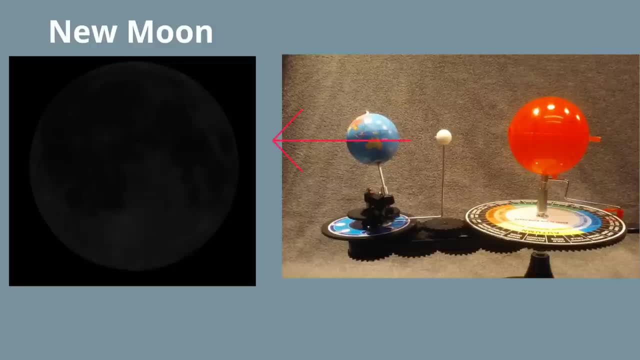 The moon cycle, or lunar cycle, begins at new moon. Here's the alignment of new moon And here's what new moon looks like from earth. And yes, it is very dark. The moon travels roughly 13 degrees in 24 hours. So after roughly three and a half days the moon has moved 45. 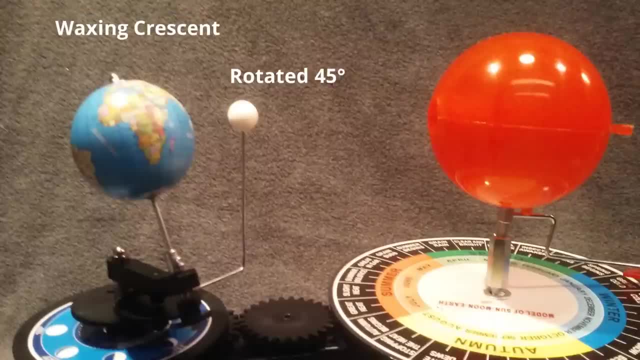 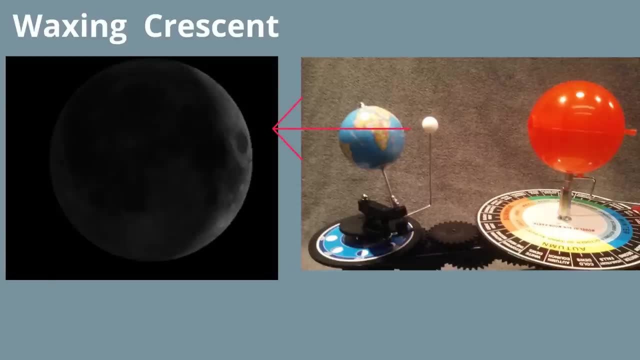 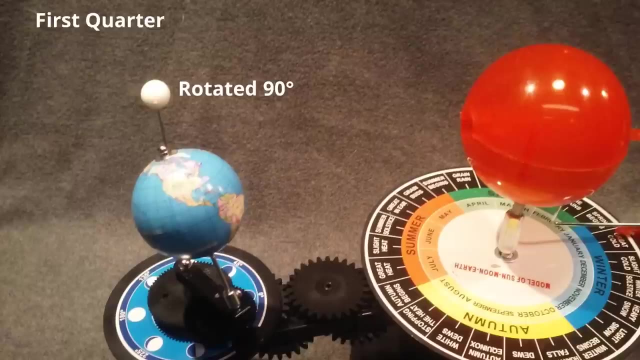 degrees and is at waxing crescent. Here's the alignment. Waxing means that the sunlight is getting larger and crescent is the shape, And here's what it looks like. In seven days, the moon has now traveled 90 degrees and is at first quarter. Here's the alignment. Remember the sunlight is. 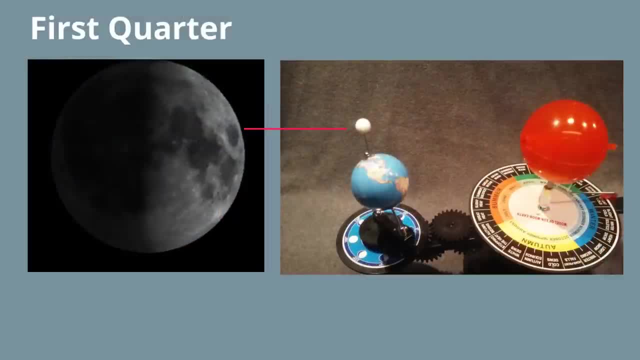 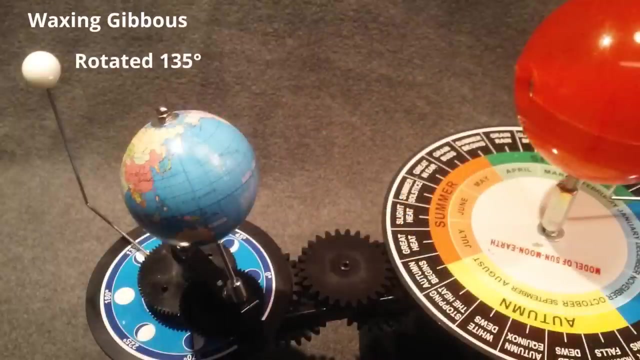 always on the right In first quarter. I remember to be first. you must be right and the light is on the right. Also, the shadow moves from right to left. In an additional 3.5 days it is now traveled 135 degrees and is at waxing gibbous. Check out this alignment. Gibbous is the shape and remember. 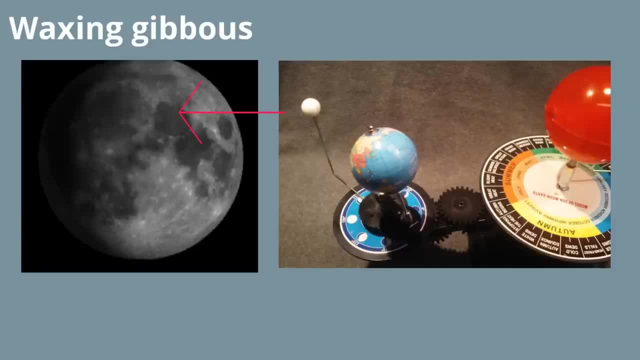 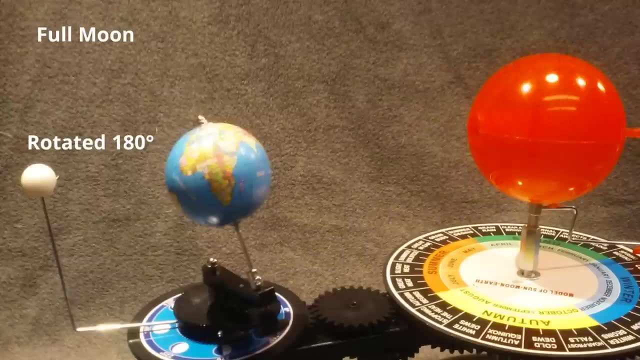 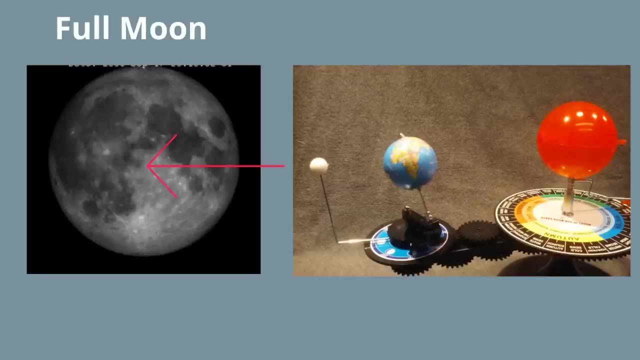 waxing means the light portion is growing. After 14 days since new moon, the moon has now traveled 270 degrees and is at full moon. Here's the alignment. And here's what a full moon looks like. After another 3.5 days, the moon is now at waning gibbous. Here's the alignment. 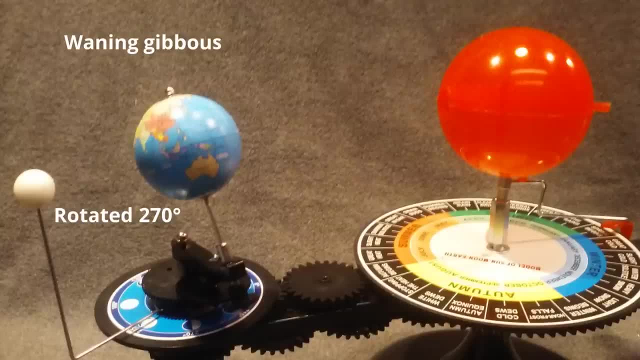 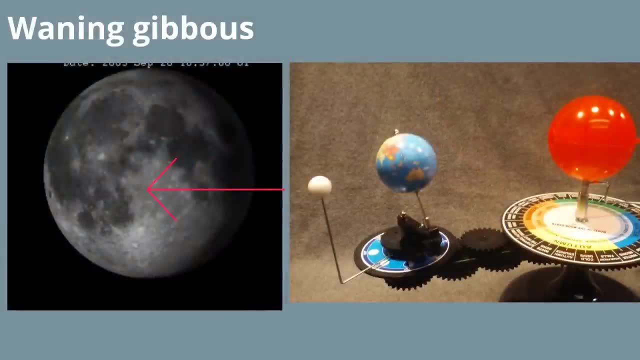 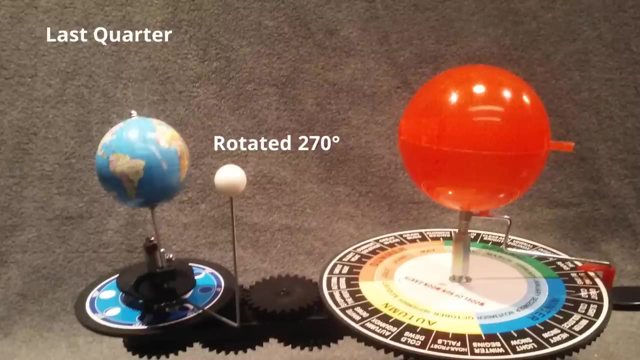 Waning means the light is getting smaller, And here's what it looks like from earth. Again, remember, the shadow moves from right to left. After 21 days, the moon has now traveled 270 degrees and is at last quarter. Here's the alignment. The light is now on the left, and I remember. 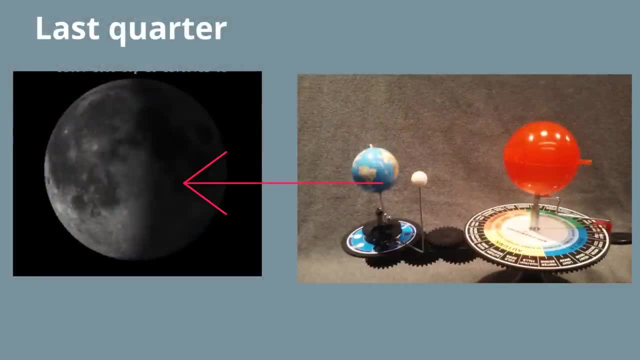 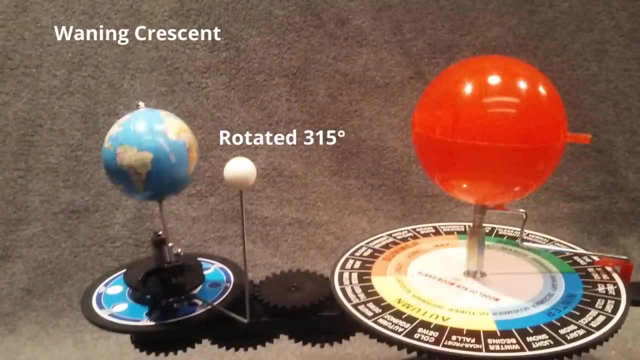 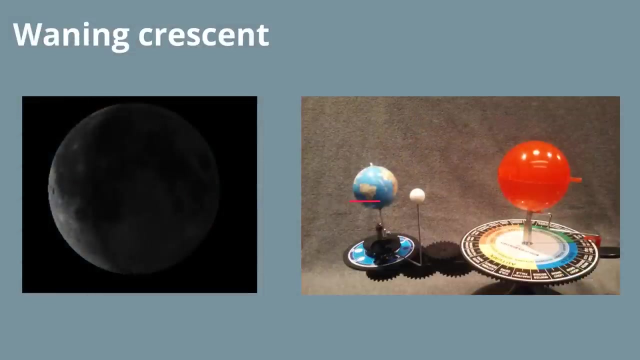 if you got last, you got left behind. After roughly 24 days, the moon is now at waning crescent. Remember, waning means the light is getting smaller And the sun, earth and moon alignment looks like this: And finally, after roughly 27 days, the moon is now back at waning crescent. 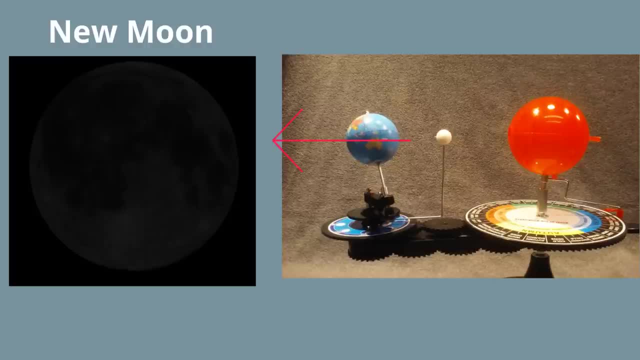 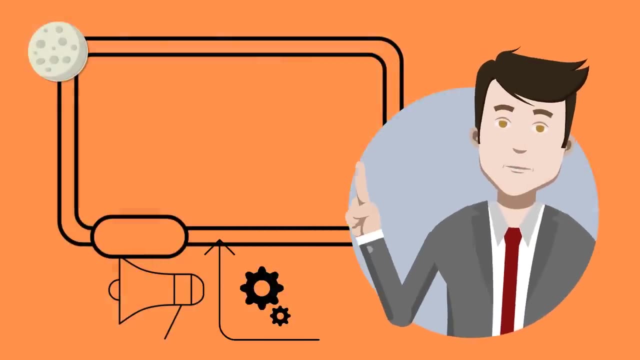 at new moon and the lunar cycle will start over again. If you would like to know more about the phases of the moon, this playlist will help. Thanks for watching. Please subscribe and share.